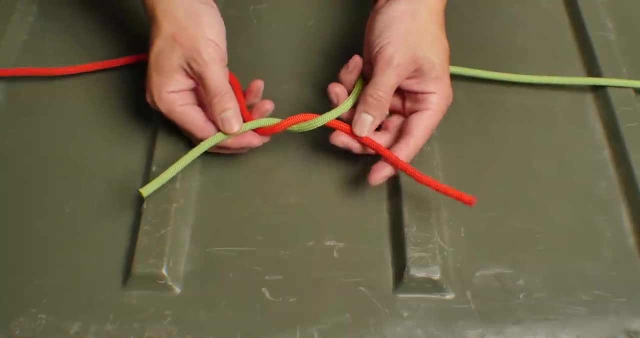 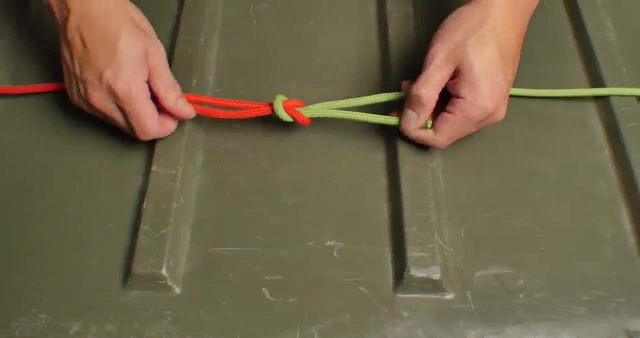 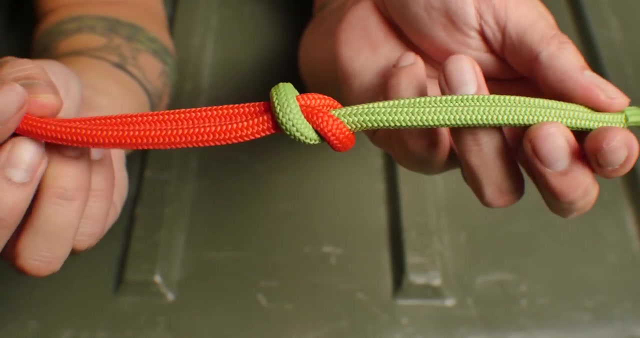 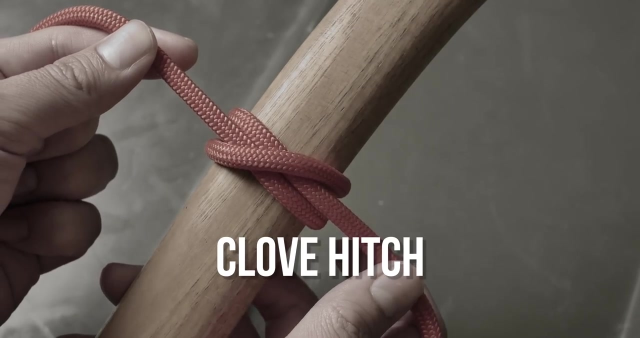 of the same rope. You go right over left for one of the knots and then left over right for the other. The result should be a symmetrical knot with two ends running parallel to each other. The second knot is the clove hitch. The clove hitch is used a lot in boating sailing outdoor. 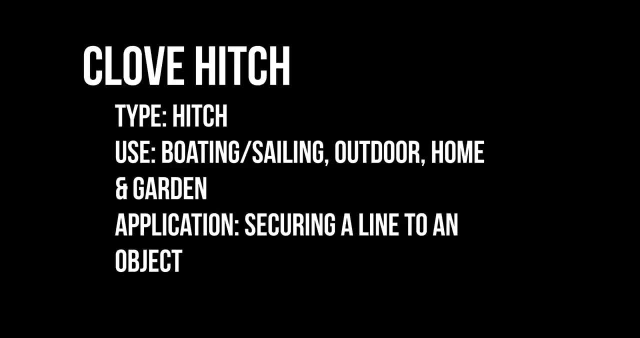 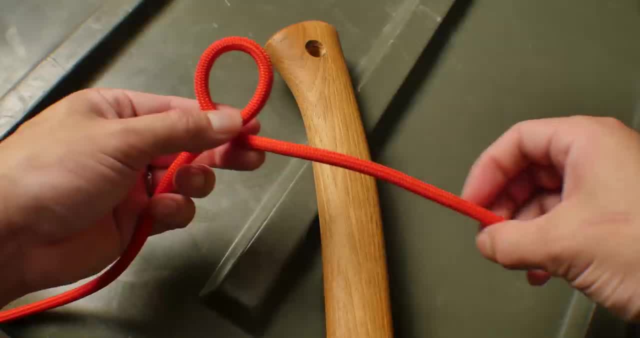 and also just around the house, And it's used for securing a line to an object. To start in the middle of the line, I take my hand and I twist the rope away from me. This forms a loop. Doing it the exact same way a second time forms a second loop. The second loop. 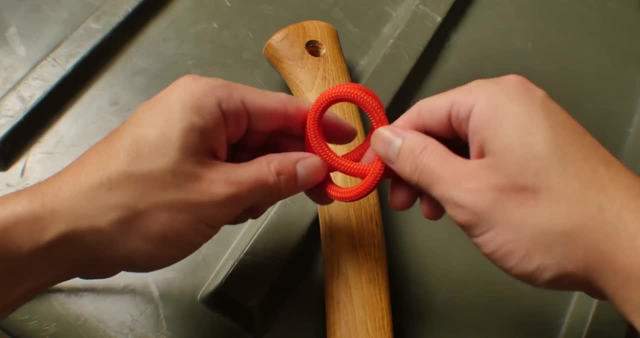 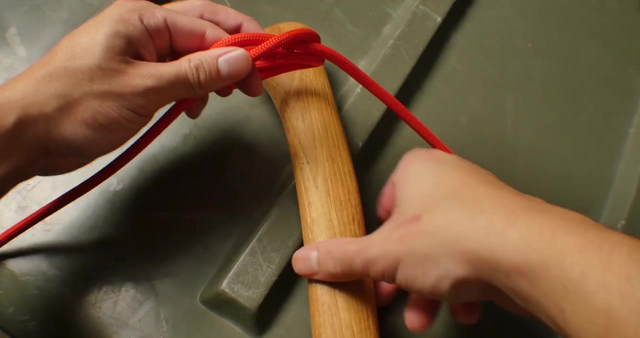 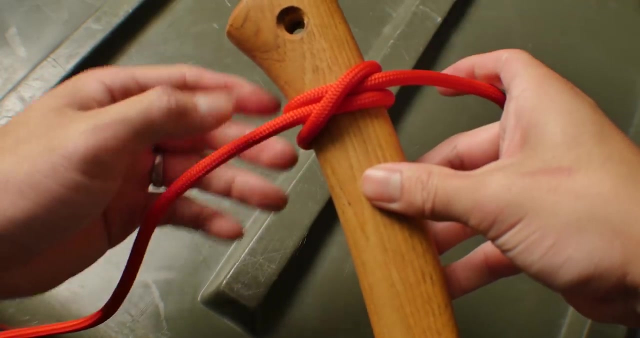 goes on top of the first loop, You'll notice that both of the ends are in the middle. The hitch is then placed over your object and can be tightened 7 Knots. You Need to Know To tie from the end. you bring the line all the way around the object below your working. 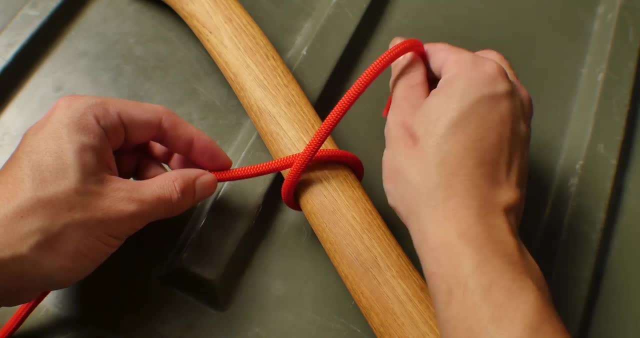 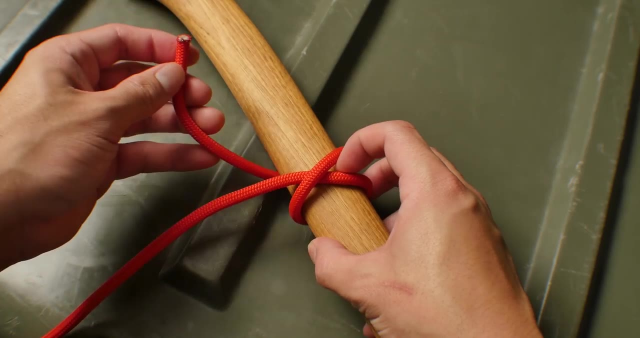 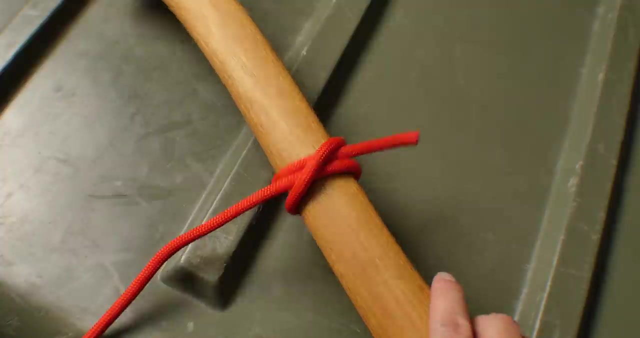 end. The loose end then goes above your working end around the object once more. The loose end is then passed underneath the overlapping line- 8 Knots You Need to Know To tie a proper clove hitch. you'll have no binding, no jamming and everything will be. 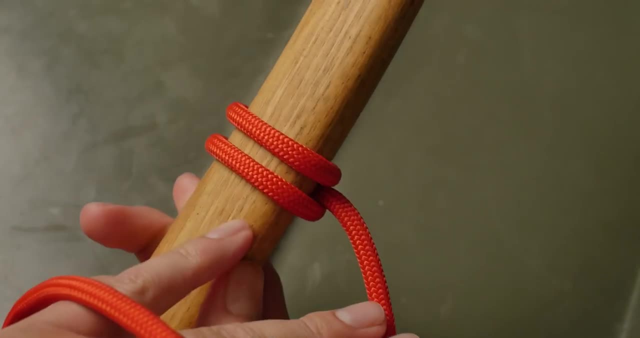 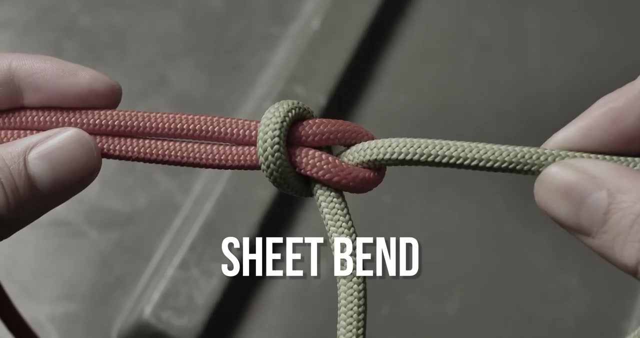 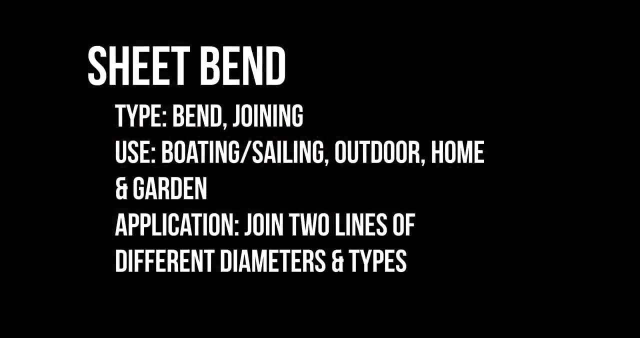 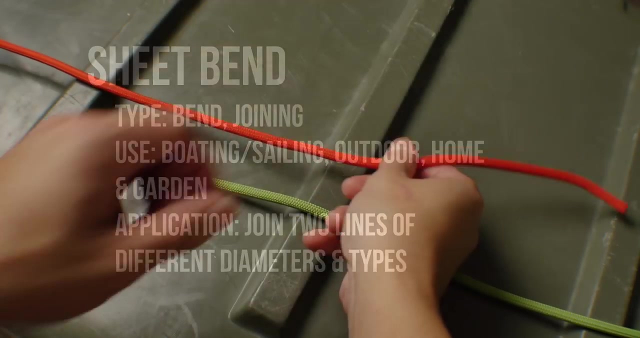 parallel to each other, receive 7 knots, And to cylinder and post it Maidenhills. The third knot is a simple sheet bend. This is a joining knot used in boating, outdoor and also around the house. The primary use for this is to join 2 lines of different diameters and types. Start with. 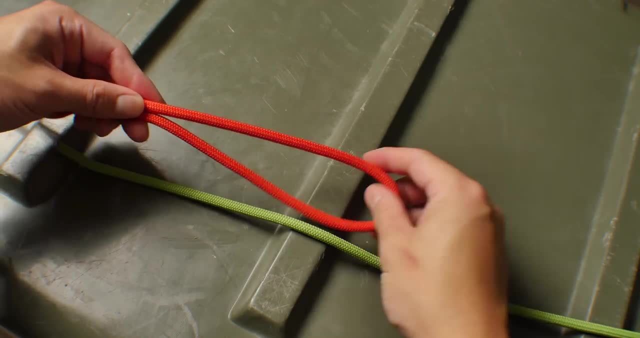 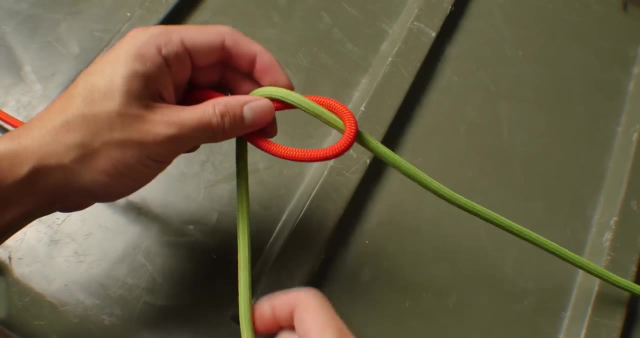 one line in a bite, 2 lines both diagonally and vertically. Just join them together. just this will be the thicker diameter of the two. The smaller diameter line will go up through the bite. It is wrapped around and then tucked underneath itself. 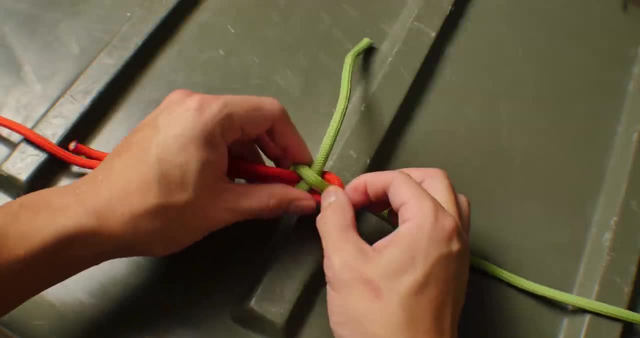 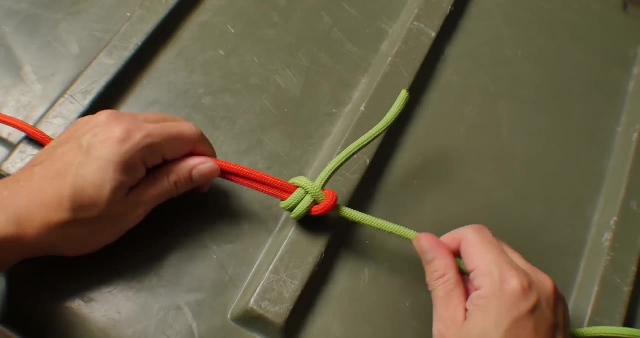 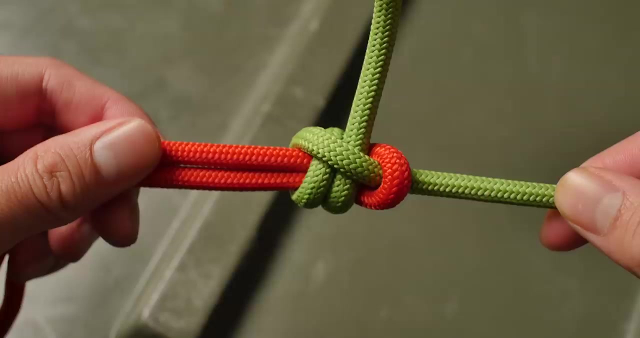 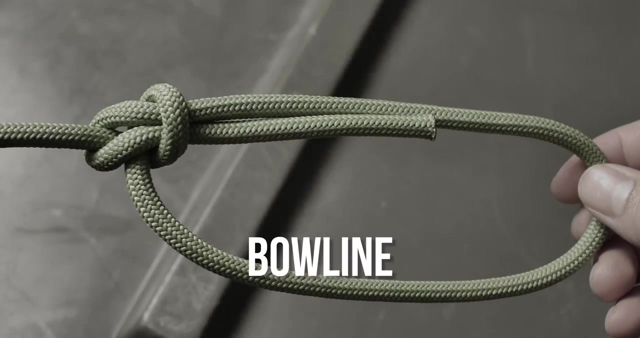 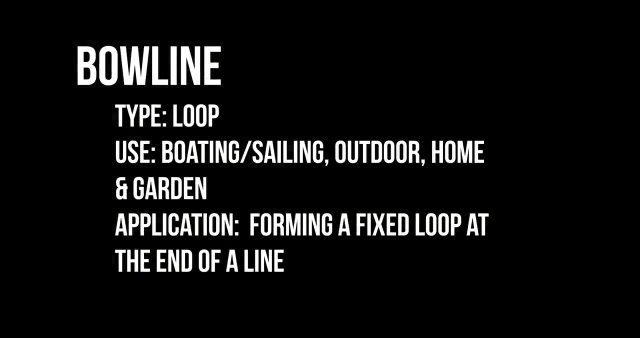 For a more secure bend. you can turn this into a double sheet bend by simply bringing it through one more time. If done properly, both of these will look very clean and will be easy to undo when you need it to. The fourth knot is a bowline. The bowline is a loop knot primarily used in boating. 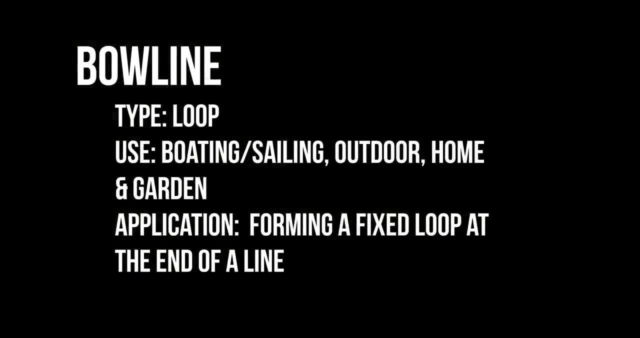 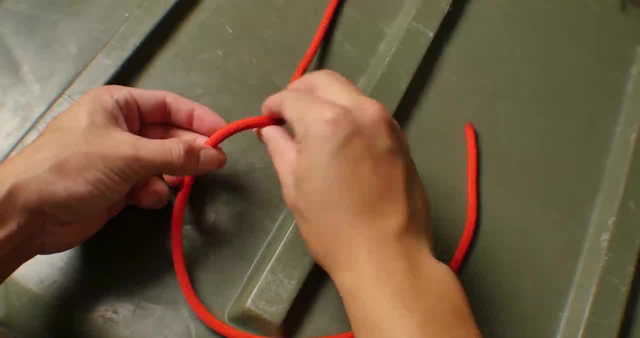 but also in the outdoors and around the house. The bowline is great for forming a fixed loop at the end of the line quickly. First start by making an overhand loop towards the working end. The loose end is then brought through the bottom. 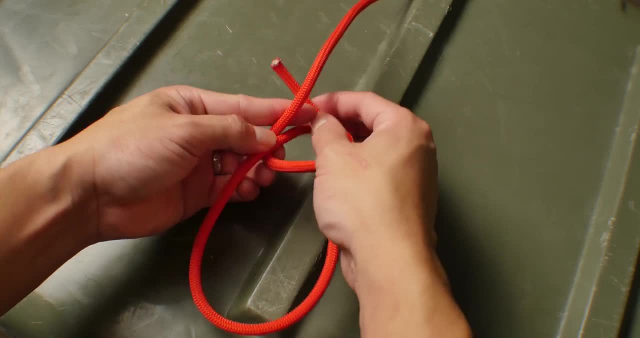 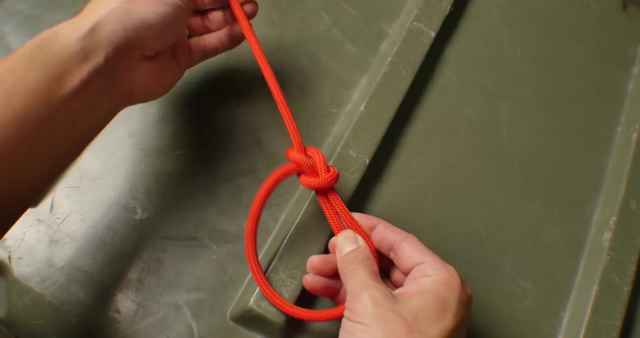 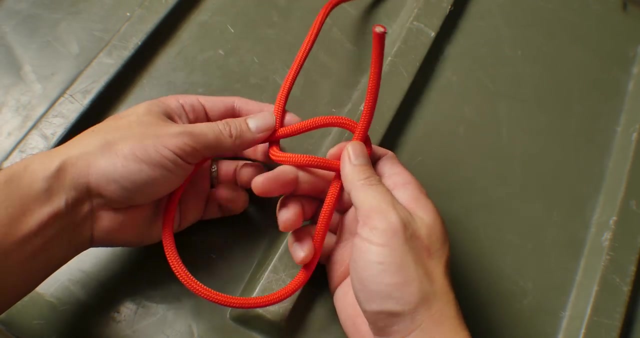 through the loop around the working end and then back through the top of the loop. To do this quickly, I swoop around the working end and rotate my wrist. This forms a loop. The line can be put around the working end, brought through the loop. 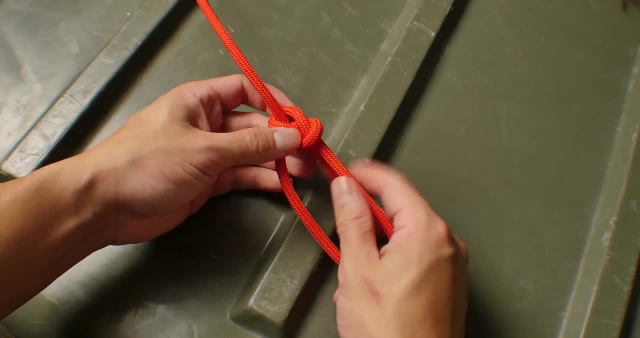 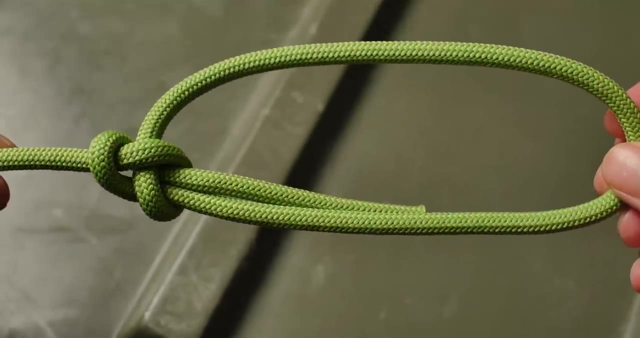 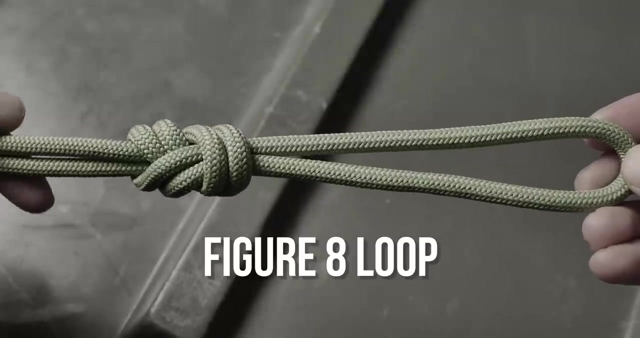 and then tightened back up. With a little bit of practice, you can do this one-handed. This is what it should look like when you're done Knot number five is the figure eight loop. This is one of my favorites because I use it a lot. 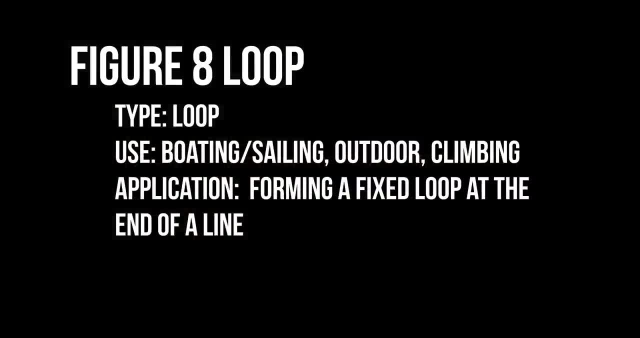 during rock climbing. The figure eight loop is used a lot in sailing in the outdoors and also during climbing as well. It is great for forming a fixed loop at the end of the line that's unlikely to slip, Starting with the bite. drape it over your hand. Snake it around the front of your hand. 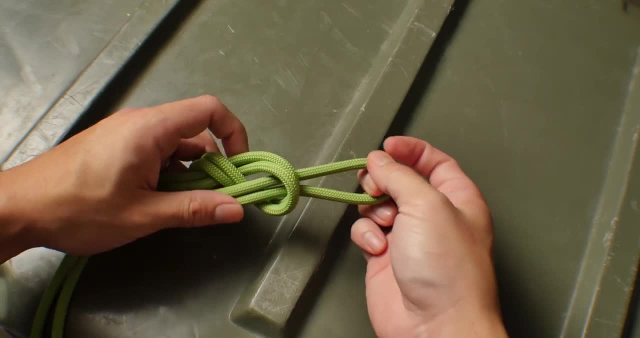 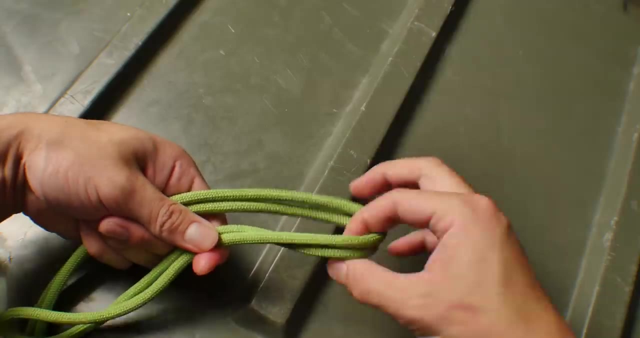 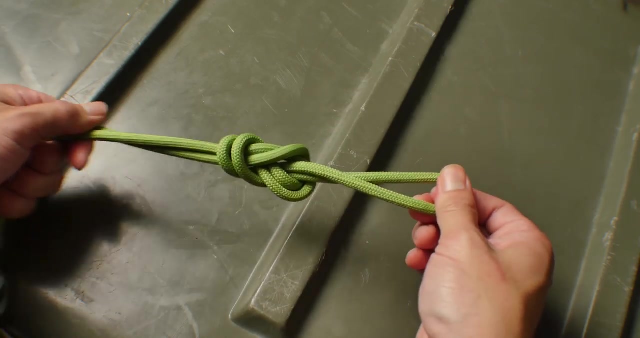 through the back and then fish the bite through the eyelet. After you finish with a little thatch of the bolt, pull it around. Another way to do this is to bend the bite and twist it two times. Bring it through the back and you've formed a figure eight. Sink, new pin, briquette, rigidelog or just Ocean Head'd- it can be a little hearts and walnut rageru know about, which also organization that located. another way to do this is to bend the bite and twist it two times, bring the back and you form a figure 8. 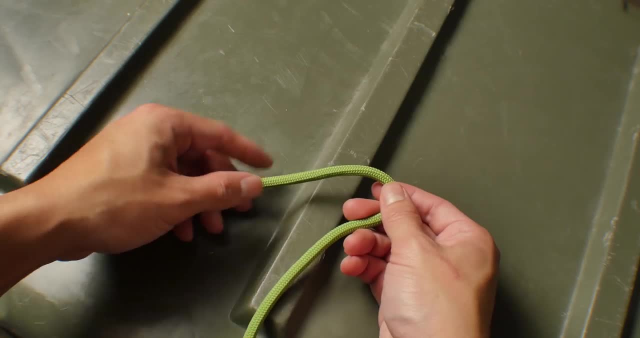 tying with bounced off. I hope you find it useful. score it. you find better ideas from everyone on this cd. If you're attaching through a fixed loop, you're going to need to do a figure eight. follow through. Start by making a single figure eight with one strand. 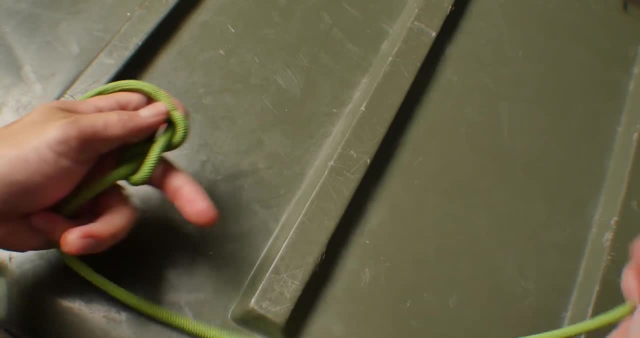 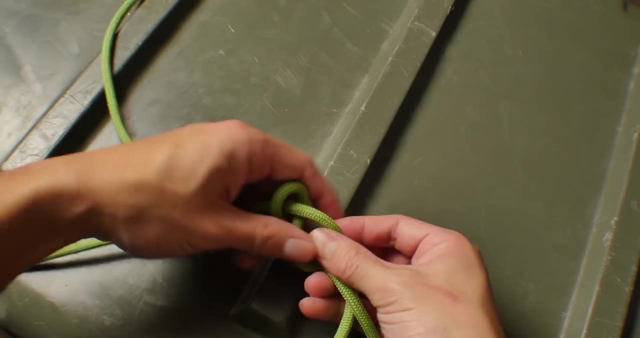 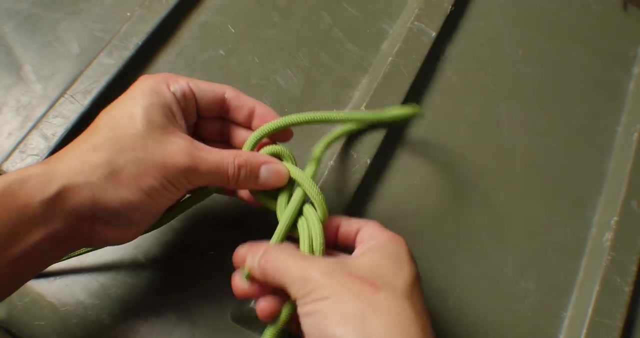 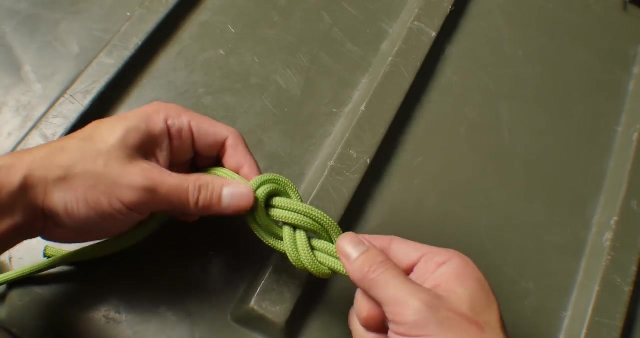 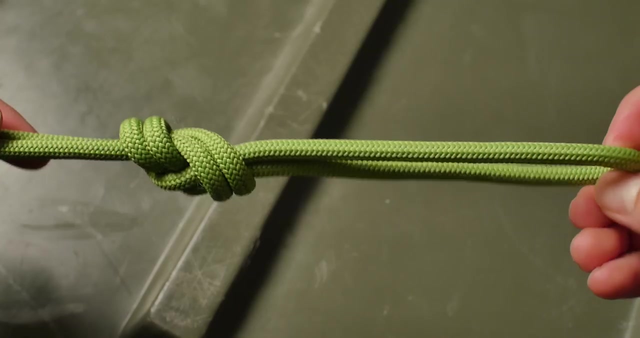 You'll bring the loose end through whatever object you're looping through, and then you'll go and retrace the exact same steps, beginning from the exit. When you're done, make sure that everything is dressed so that everything lays nice and flat. The sixth knot that we're going to do is a round turn and two half hitches. 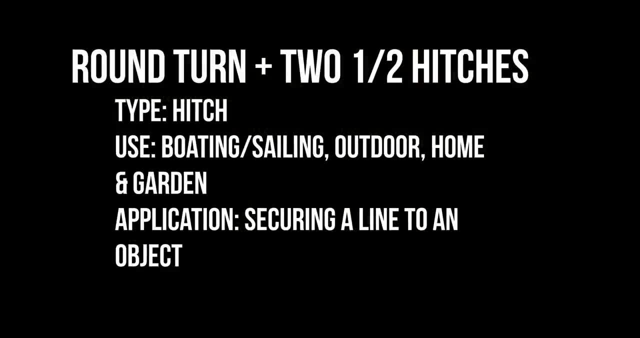 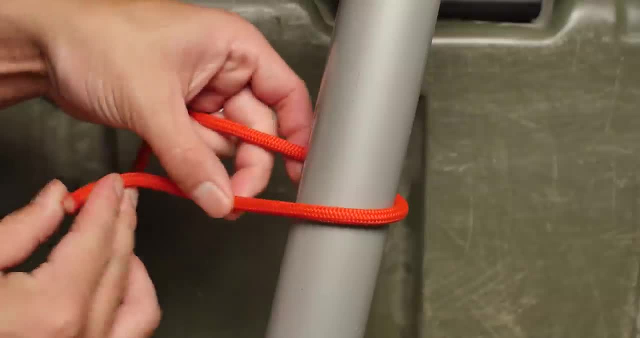 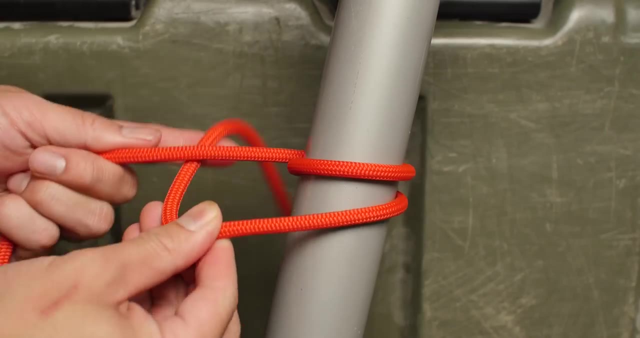 This is a hitch primarily used in boating, but is often seen in the outdoors and also around the home and garden. It's primary use to secure a line to an object. We'll start by doing the round turn. The loose end is then brought underneath, over the working end and through the loop that it forms. 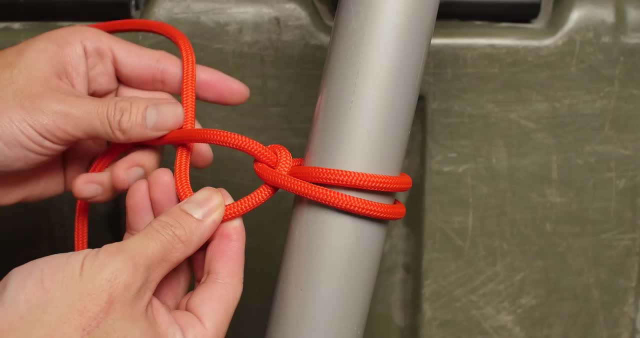 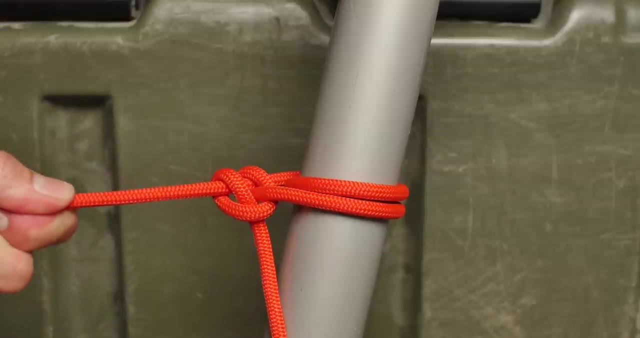 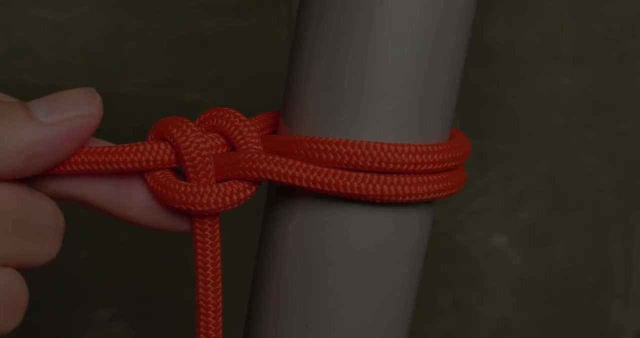 This is one half hitch. You need to do this again for the second half hitch. I saved my favorite knot for number seven, the taut line hitch. The taut line hitch is an adjustable loop used a lot in boating, outdoors and home and garden. 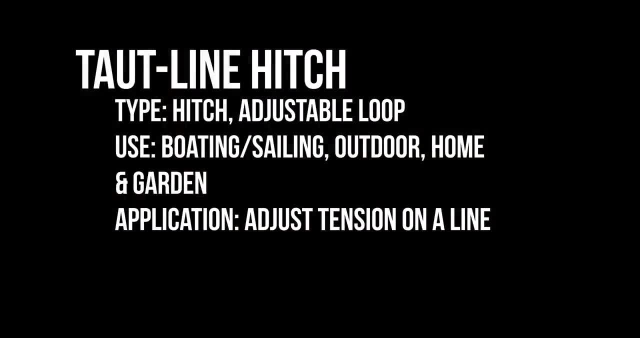 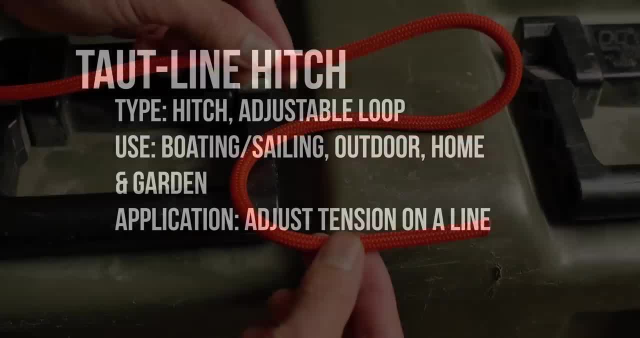 Its primary function is to adjust tension on the line. Fish the non-working end through. whatever you're going to be attaching to For the first half hitch, you're going to need to make sure that everything is dressed. You'll bring the loose end through whatever object you're looping through. 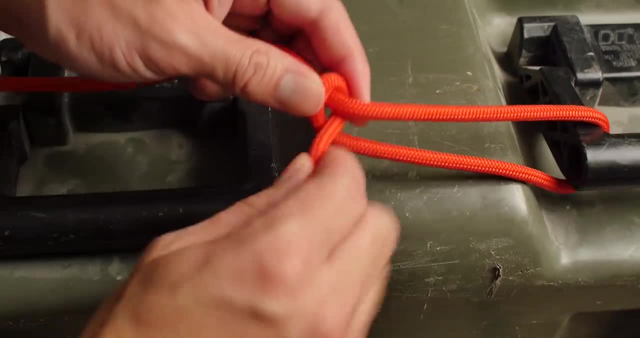 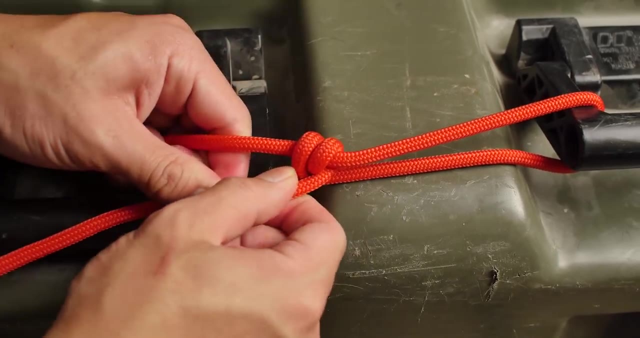 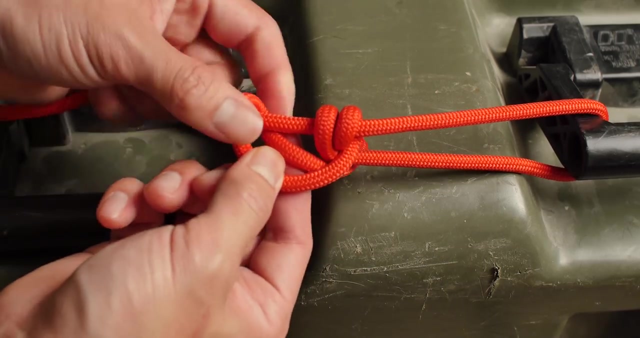 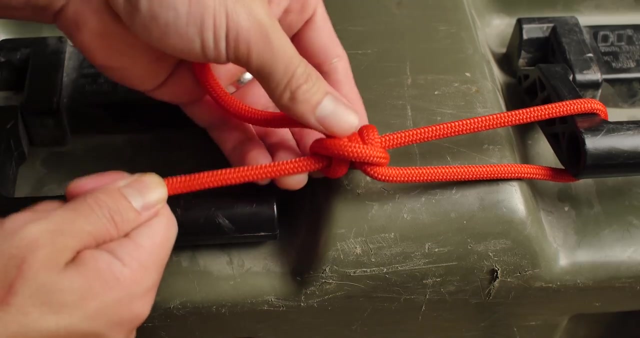 Form a loop and do two passes on the inside of that loop Going the same direction. form another loop and then pass it through. You know you've done this right. when the loop goes one way and you're trailing out, The loop at the end goes the other way. Loosing and tightening is as easy as grabbing the knot and sliding it around.